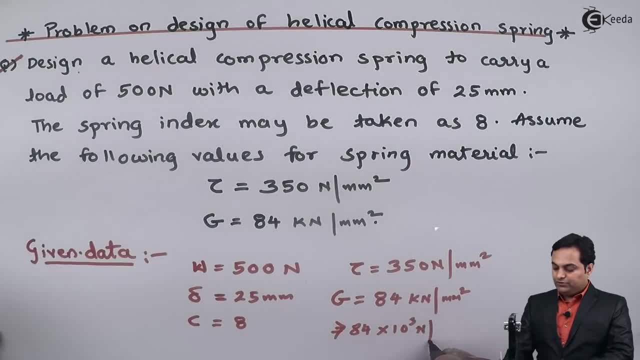 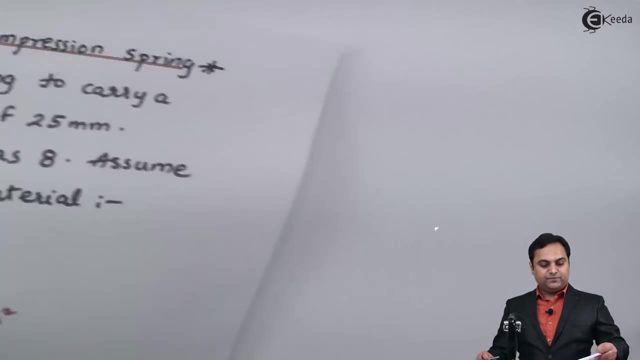 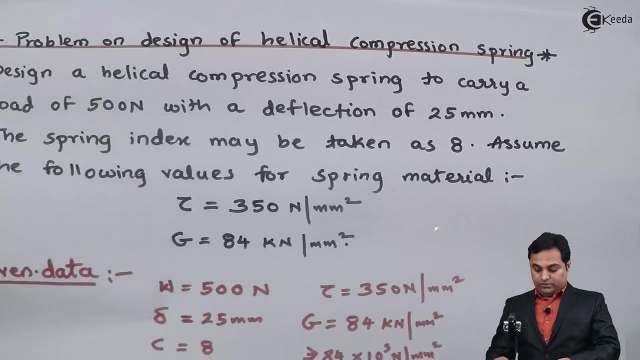 84 into 10, raise to 3 Newton per mm. square. now for these data available, let us try to design the spring. so, in the solution for this problem, since the value of load and deflection they are given, The first thing which I can calculate is this: 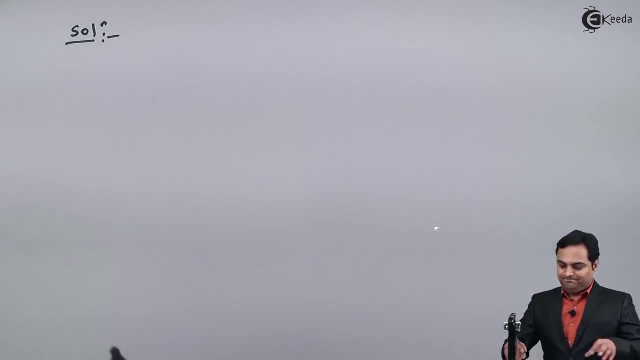 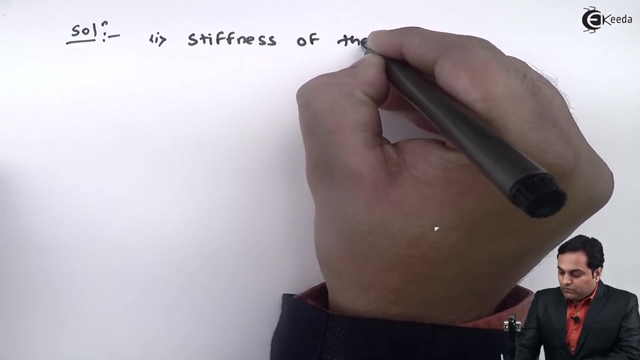 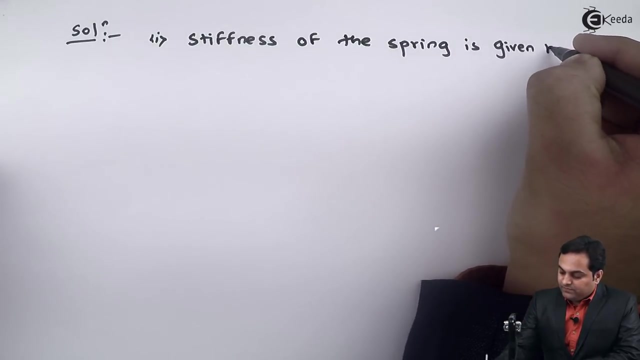 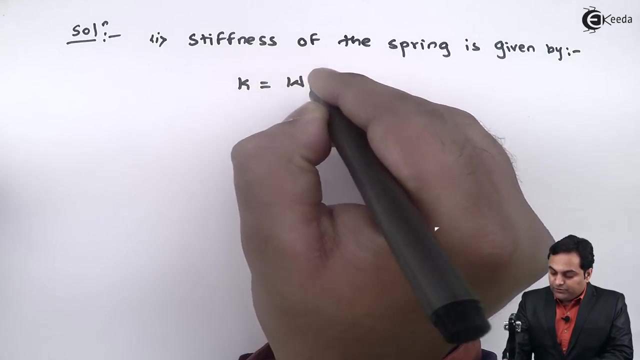 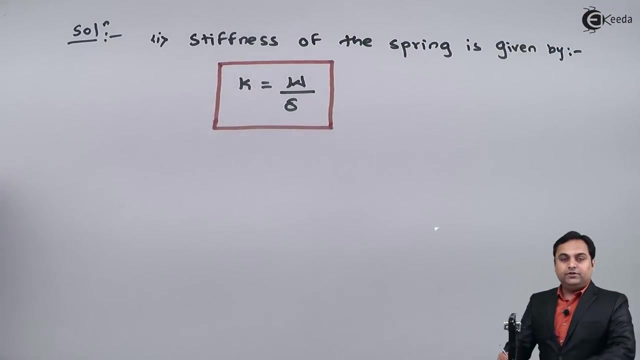 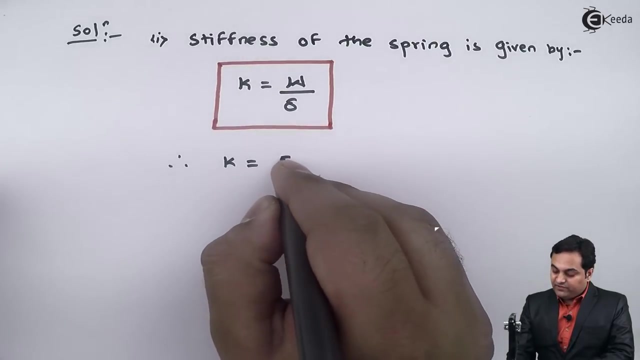 calculate. here is the stiffness of the spring. so here I'll write down: stiffness of the spring is given by. stiffness is denoted by capital K, and that is equal to load upon deflection. here I'll put the values: K is equal to load, it is 500, deflection is 25. so here I get the. 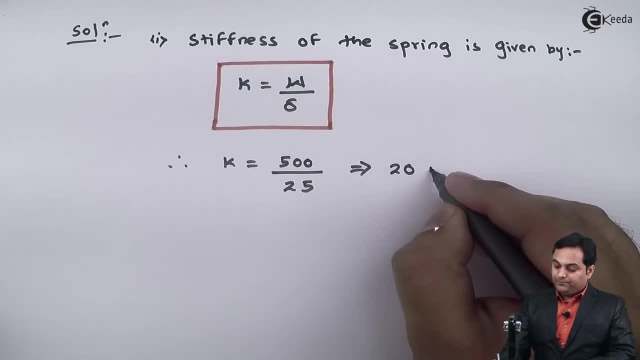 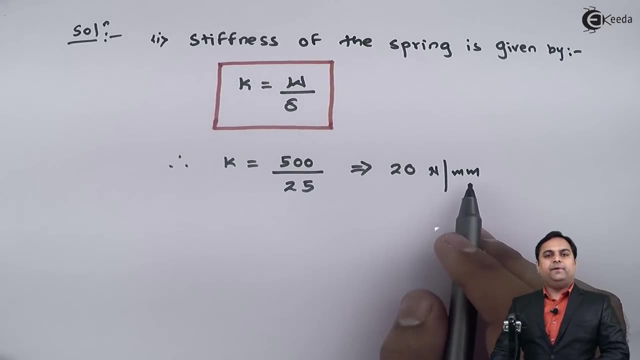 stiffness as 20 Newton per mm, so the spring will deflect by 1 mm. so this spring will deflect by 1 mm, and this spring will deflect by 1 mm. so here I get the stiffness as 20 Newton per mm, so the spring will deflect by 1 mm. 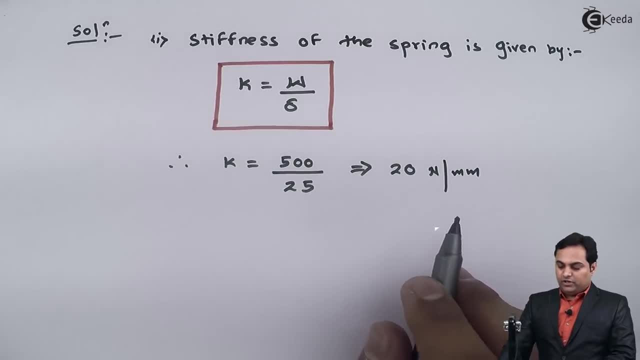 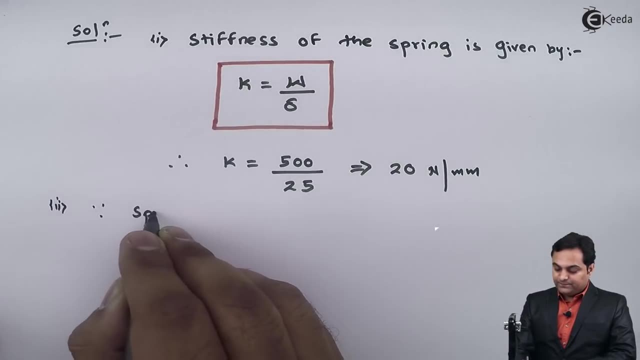 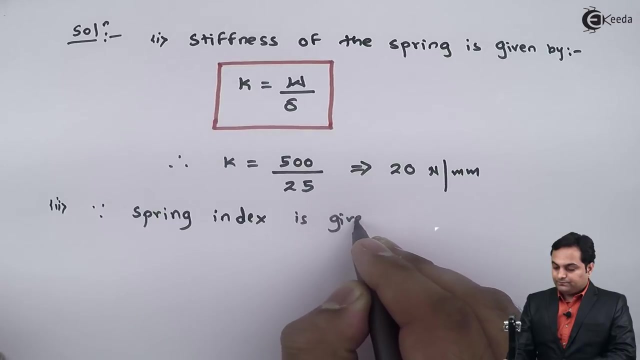 when the load on the spring is 20 N. Now, after getting the stiffness, I will write down: since spring index is given by spring index is capital C and that is equal to capital D upon small D, where capital D it is called as mean coil diameter and small d is called as wire diameter. 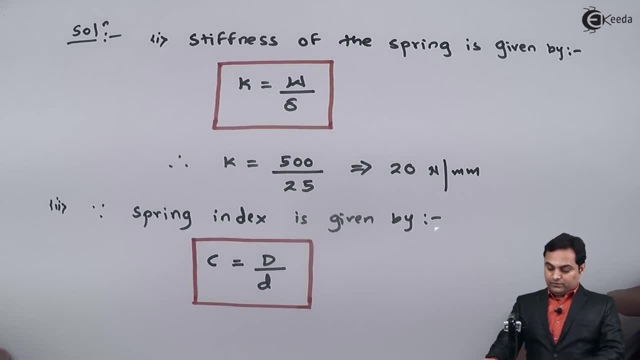 This is the formula Now. from this I can say that therefore, the value of capital D or small D, if I am able to get any one of them, I can get the other value, because C spring index is given in the problem as 8.. 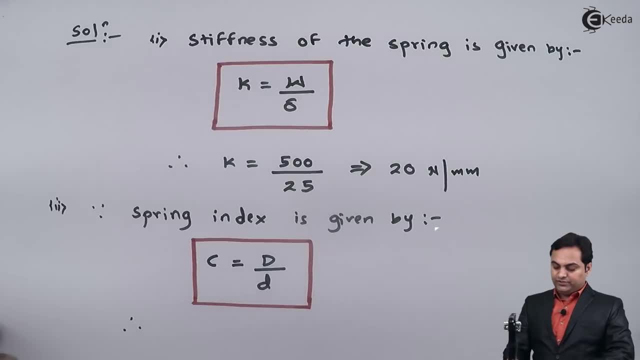 So if you know any one of the values, you can calculate the other values. So here I write down: therefore, capital D will be C into small d. I will keep this as my equation number 1.. Once I know the value of small d, I will put it in equation 1 to get the answer of capital. 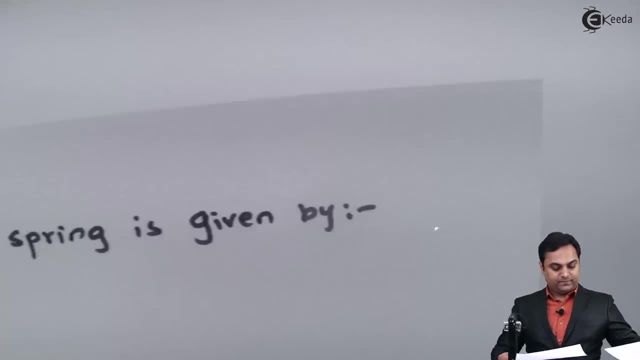 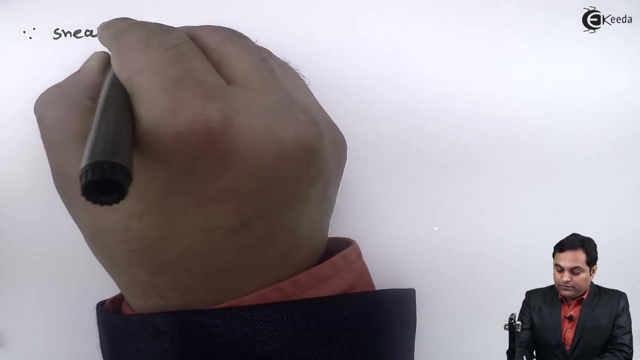 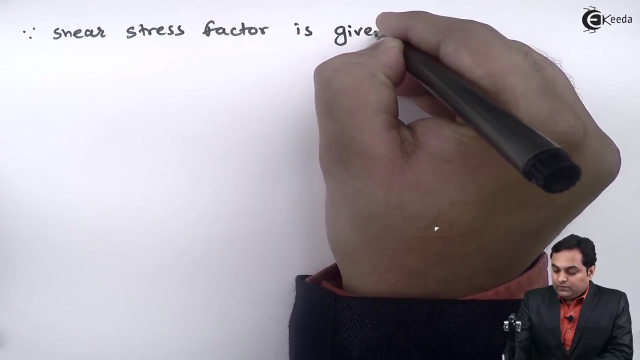 D, Next, Next Now, in this problem, as shear stress is given, tau is equal to 350 Newton per mm square. So here I will calculate the shear stress factor, since shear stress factor is given by C, So I can write down the shear stress factor. 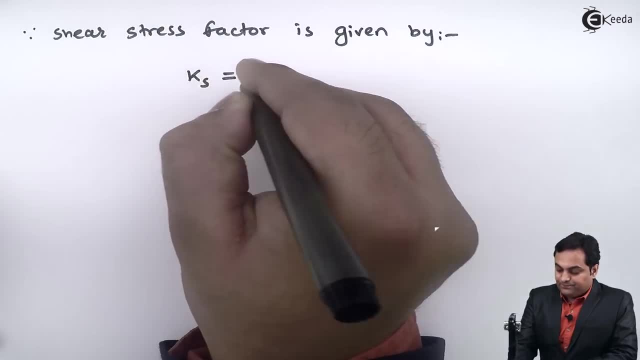 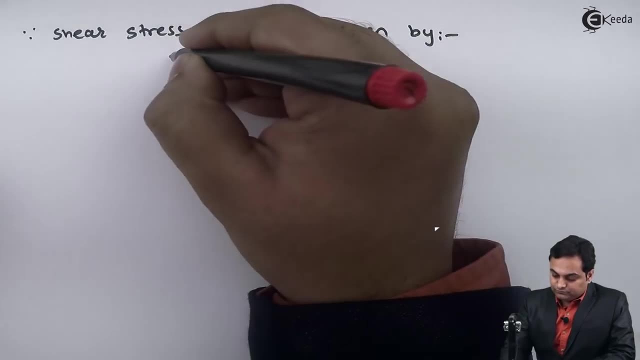 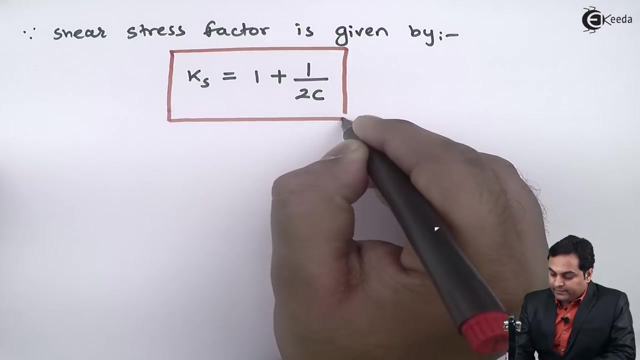 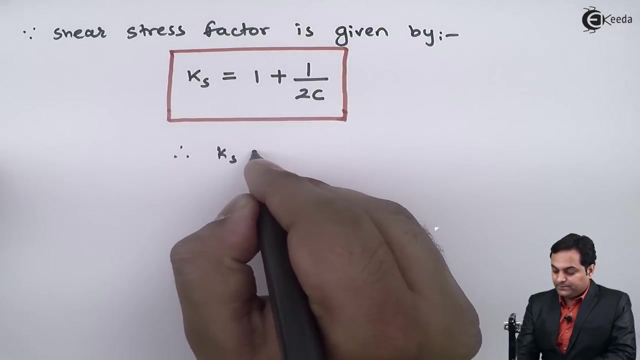 K suffix S is equal to 1 plus 1 upon 2 C. So this is the formula of shear stress factor And in this problem, as the value of C is given, I can find out K suffix S, that is 1 plus 1. 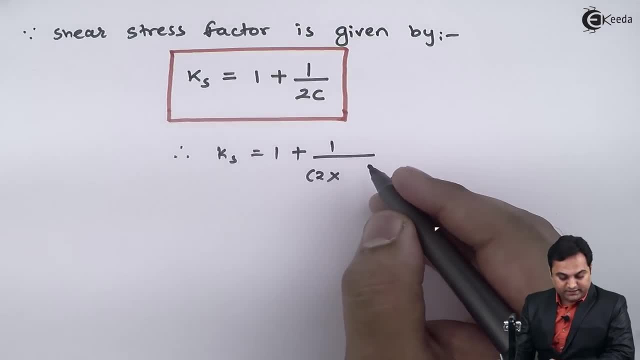 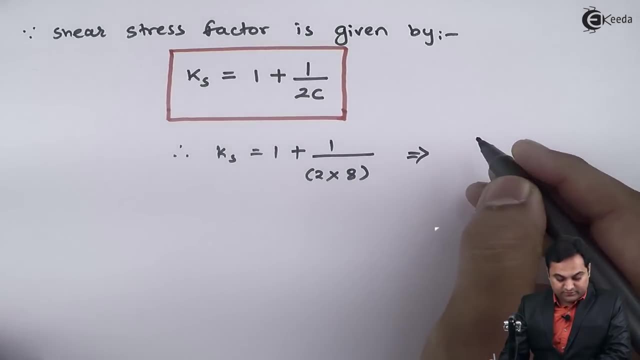 upon 2 C into C, that is 8. so if I calculate from this the answer of shear stress factor, it comes out to be 1.0625. now, after getting the shear stress factor, I can use the formula of resultant shear stress, because this tau value, which they 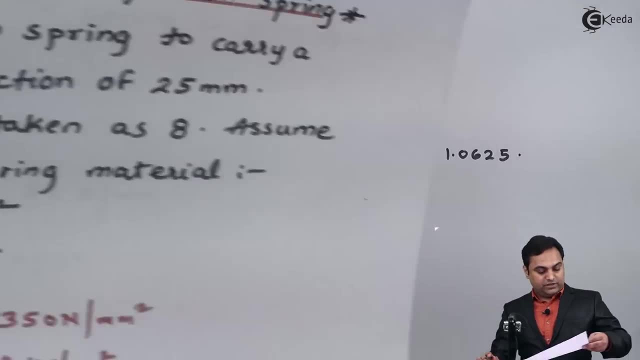 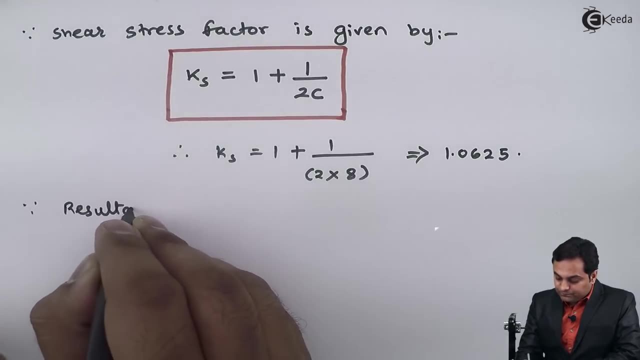 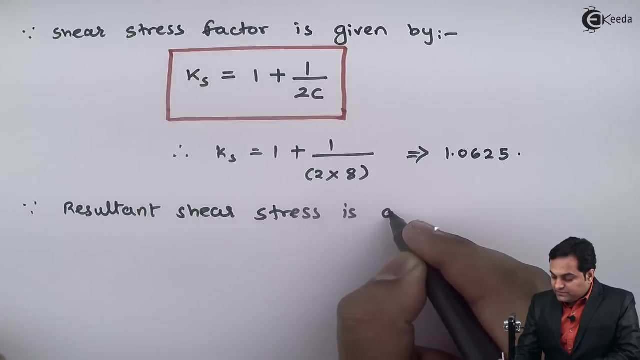 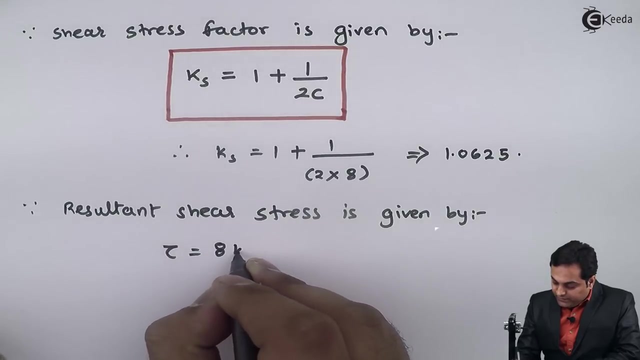 have given in the problem. it is the resultant shear stress. so I'll write down, since resultant shear stress is given by the formula is: tau is equal to 8 WD upon PI D cube multiplied by KS. this is the formula of resultant shear stress factor. I am getting the formula of resultant shear stress. 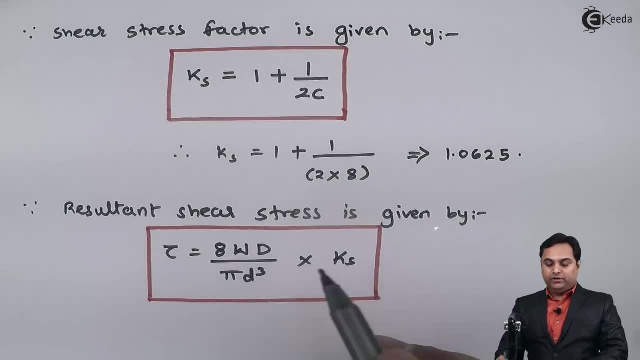 now, here, as I can see in this formula, there is one relation of D, D means D, d, that is mean coil diameter upon the diameter of wire. that is equal to C, which is spring index. So here in this formula I can simplify it in one more way, that shear stress will be equal to: 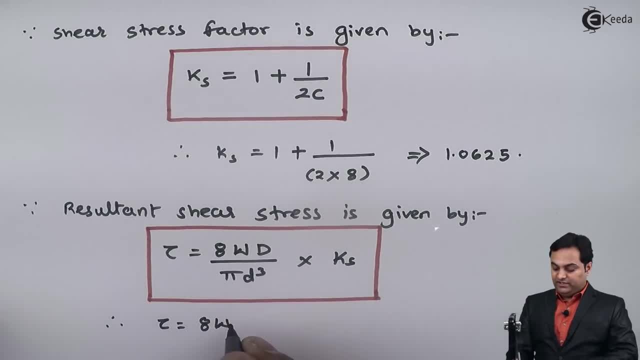 8 W. capital D upon small d is C, so in the denominator there is pi and d square will be left into ks. I will write down into the bracket, since C is equal to capital D upon small d. Now if I look into this equation, shear stress is given in the problem as 350. 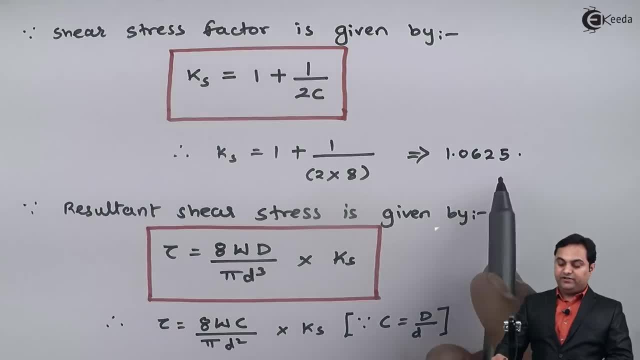 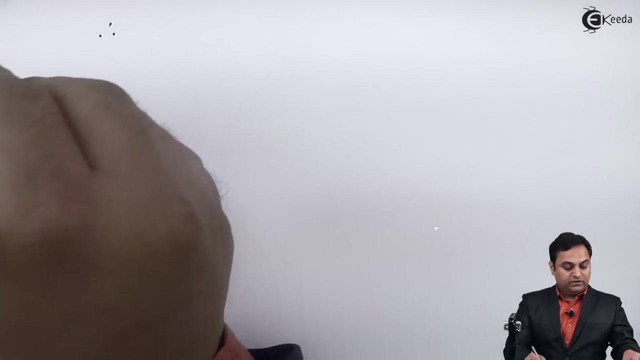 load is there spring index and shear stress factor. we have calculated just now, so only unknown. which is left is d square, which is the mean coil, which is the diameter of wire, small d. so here I will write it down as therefore shifting d square on one side. 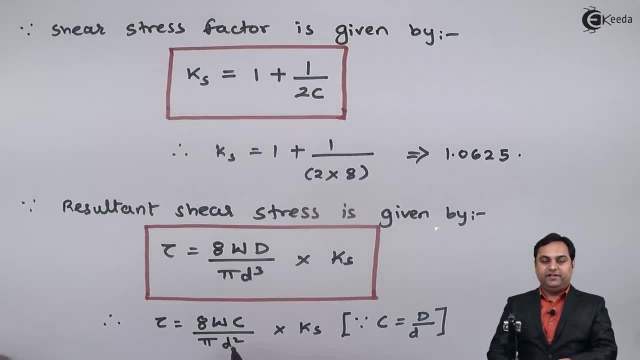 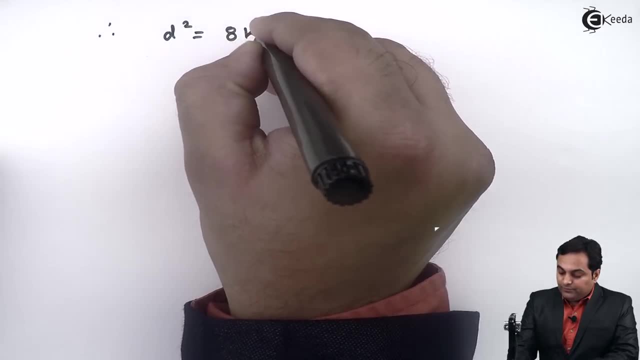 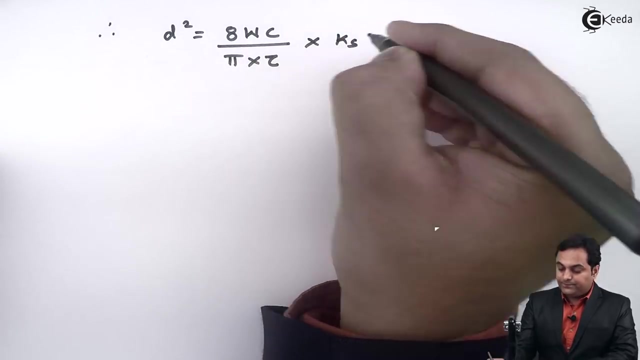 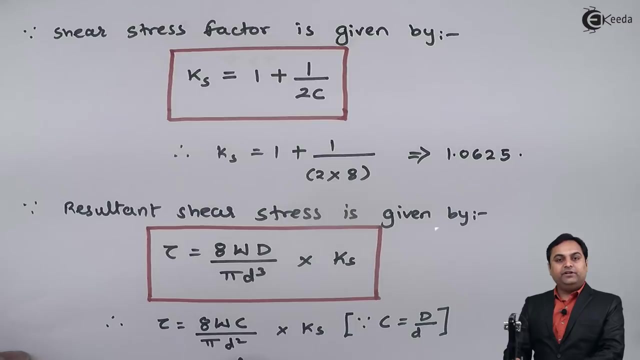 I will shift this term because I want to calculate d, so d square will be equal to 8 W C upon pi into tau multiplied by ks. here I have shifted d square on left hand side. tau will be here in the denominator on right hand side. so now I will just go on. 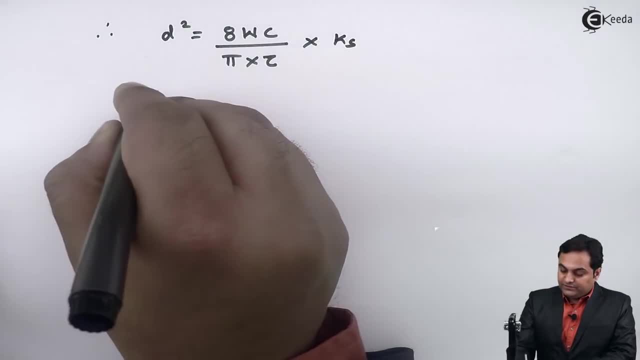 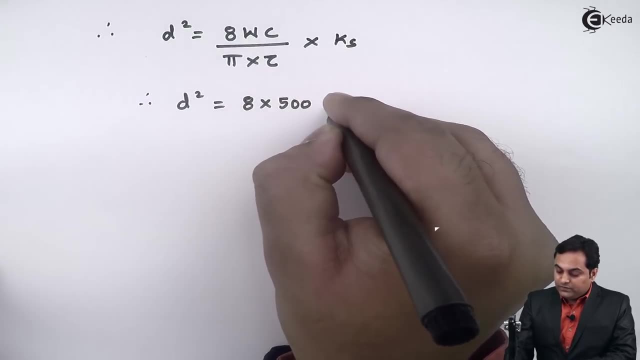 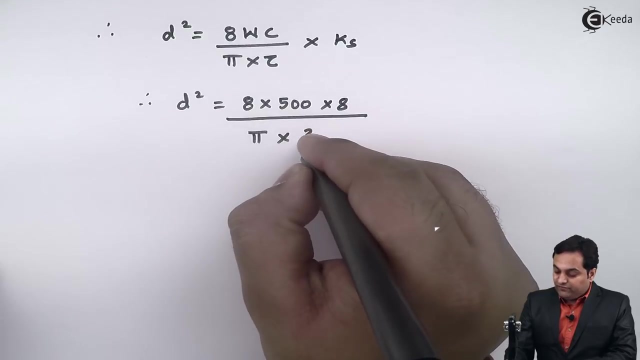 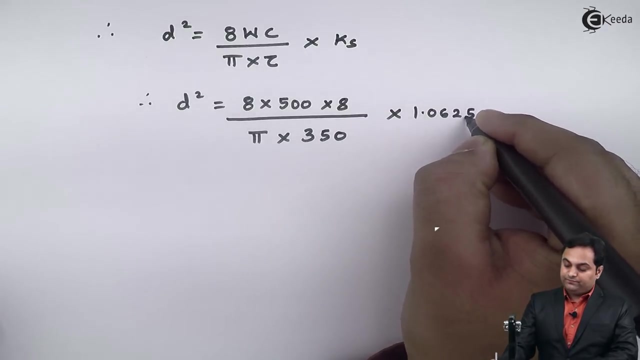 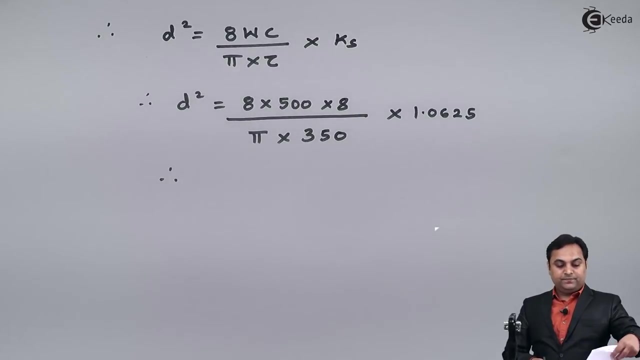 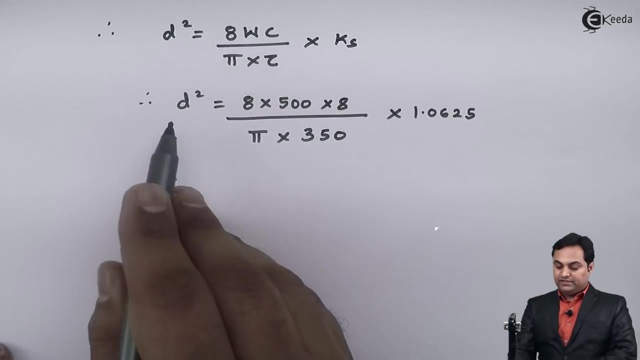 putting the values, that is d square will be equal to 8 into W is 500, C is 8 W upon pi. into tau, it is 350 multiplied by ks. shear stress factor was 1.0625. therefore, now, from this, if I calculate here, I will get an answer, and if I take the square root of that answer, 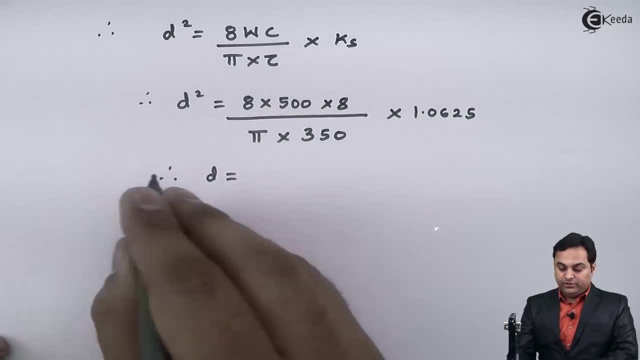 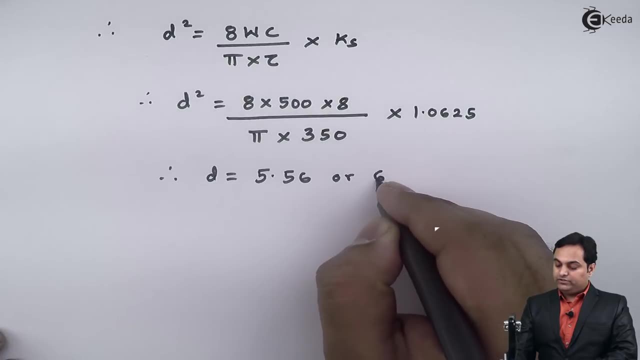 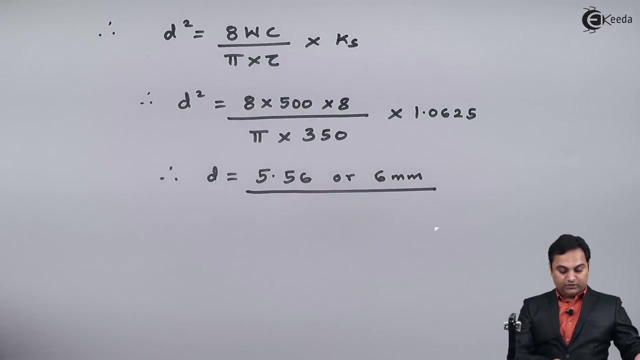 I will get the value for d and small d value. it comes out to be 5.56. I can round off this value. I will say that, or this is 6 mm. so now here, after getting the value of small d, this will be our answer number 1, that is. 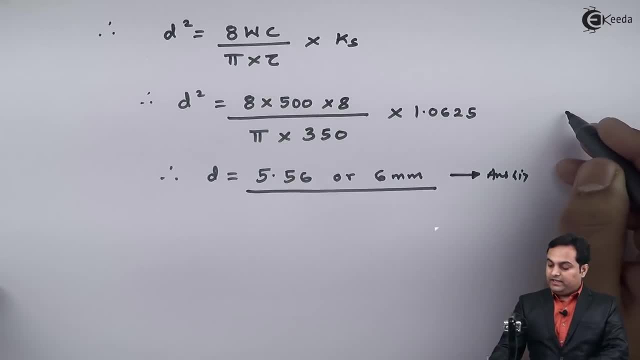 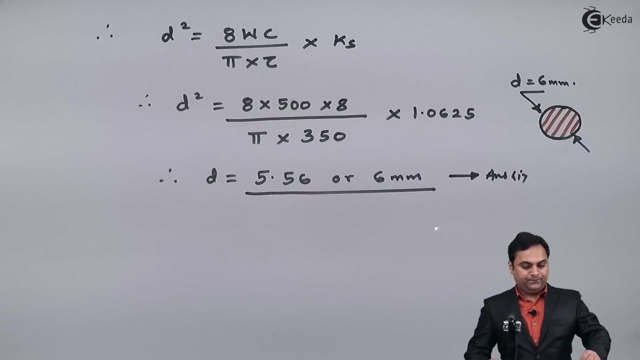 here we have designed how much should be the wire diameter, and its cross section will be circular. and here this is the wire diameter denoted by D. its value is 6 mm. now, after getting the value of small d here, I'll put this value in equation number 1 and I'll get the value. 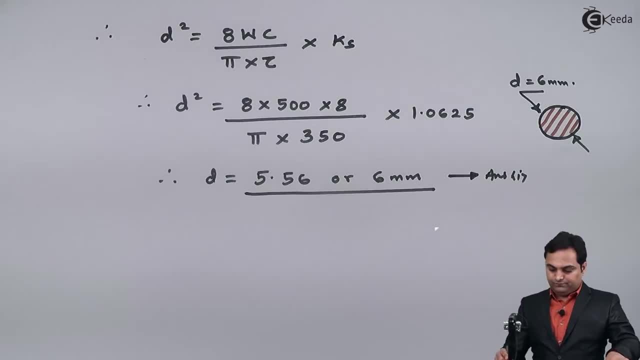 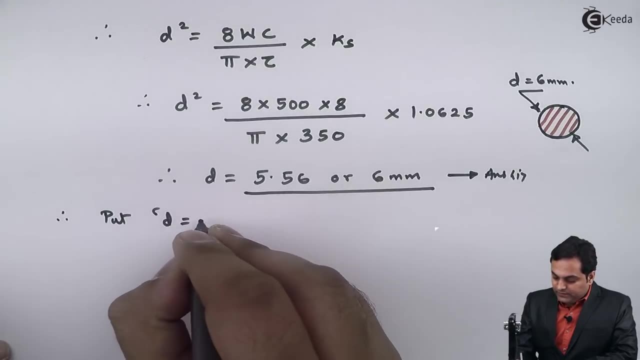 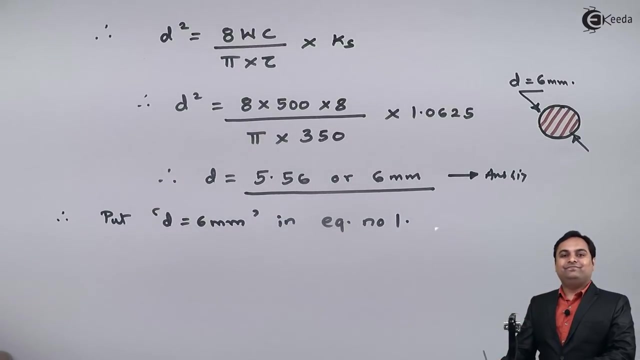 of capital D, therefore 0.. stroke point 0.. error 0. 0.. put small d is equal to 6 mm in equation number 1. so therefore we have capital D is equal to C into D, C is 8 and small d is 6. so here I get the value of capital. 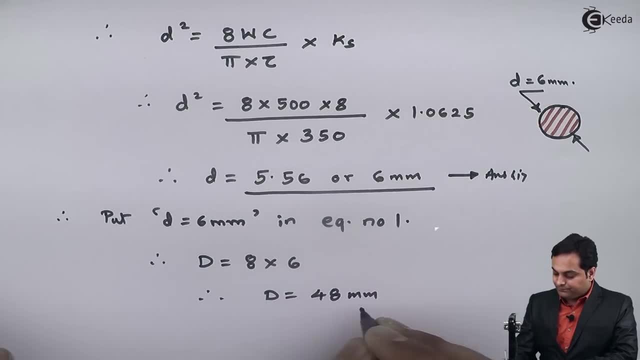 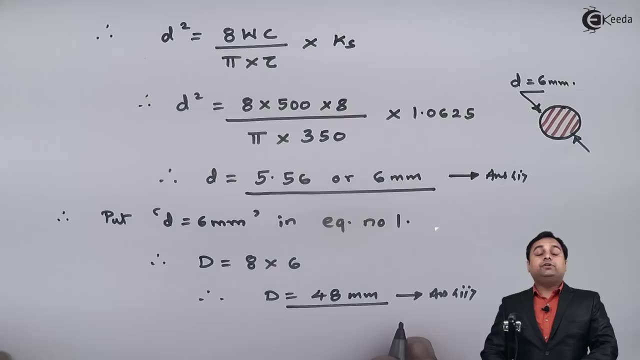 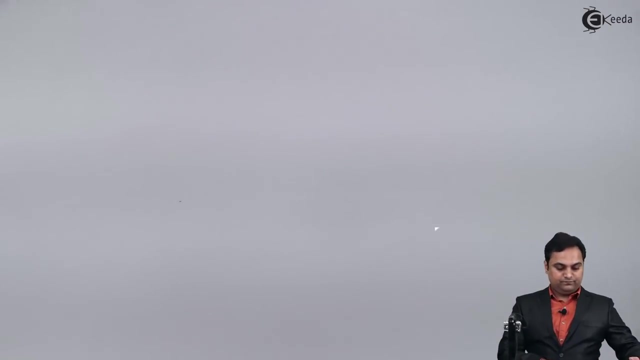 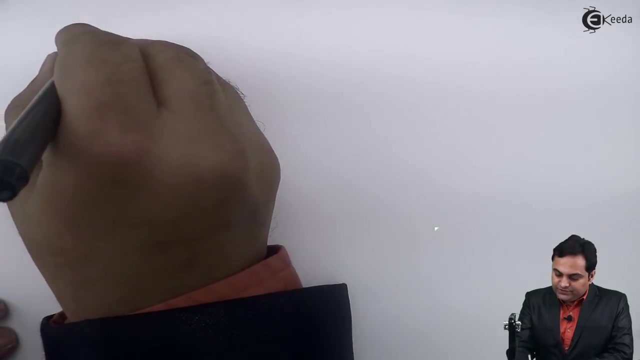 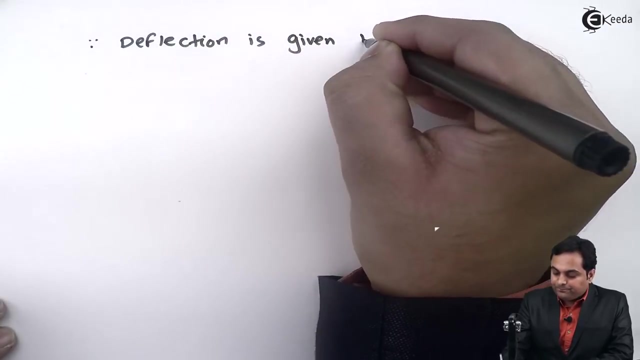 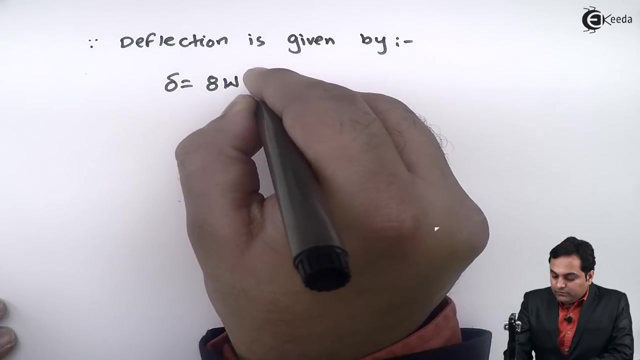 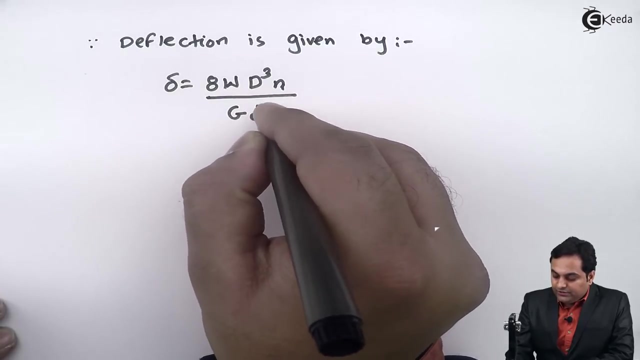 D as 48 mm. this is our second answer. so here I have got the mean coil diameter. next, after this, I'll use the formula of deflection to get the number of turns which are there in a spring. I'll write down, since deflection is given by 8 W d cube n upon G D raised to. 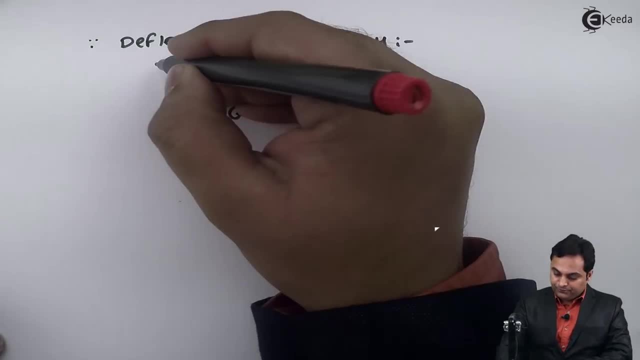 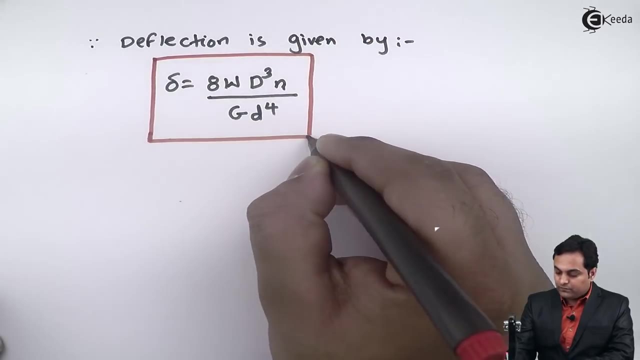 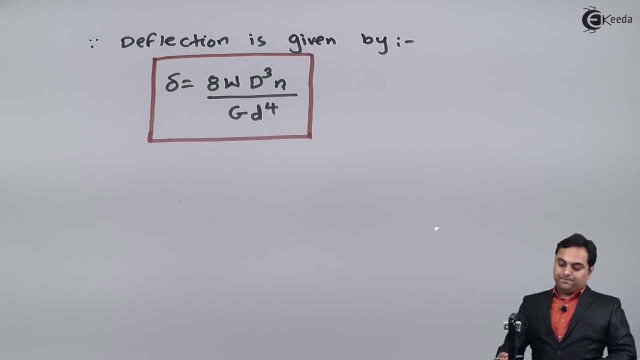 4. this is the formula of deflection. now again, in this formula, what we can do is that either we can put the values of capital D or small d, or we can write the formula in the form of small C, which is the spring index. so even if I simplify this, I'll get it, as deflection is equal. 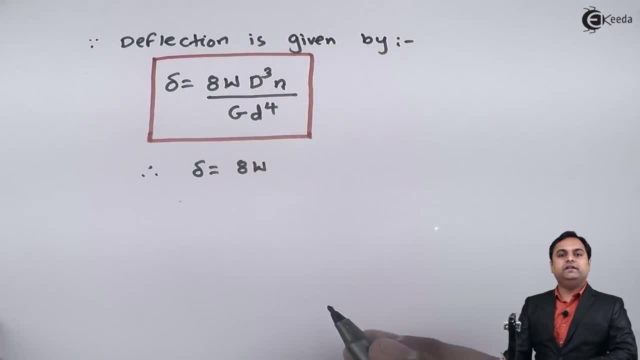 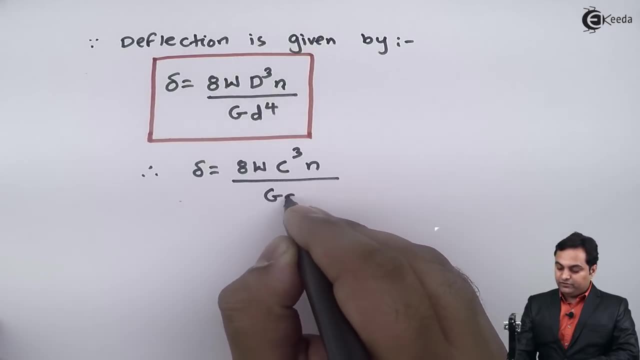 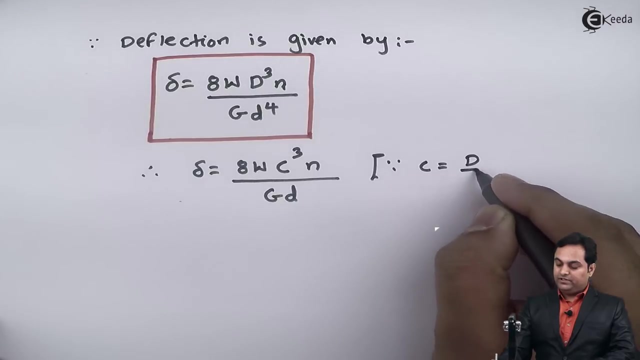 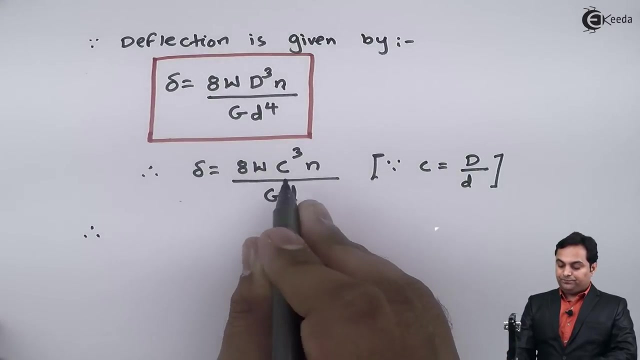 to 8 W. capital D upon small d is spring index. so spring index C is equal to 8 W cube into n upon. here I am left with only g into D, into bracket, since capital C is equal to capital D by small d. so therefore here I want to calculate n that 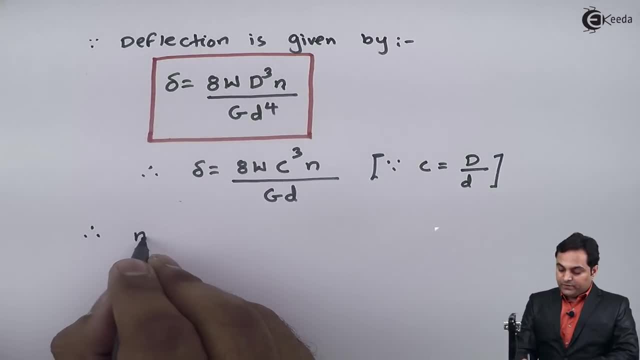 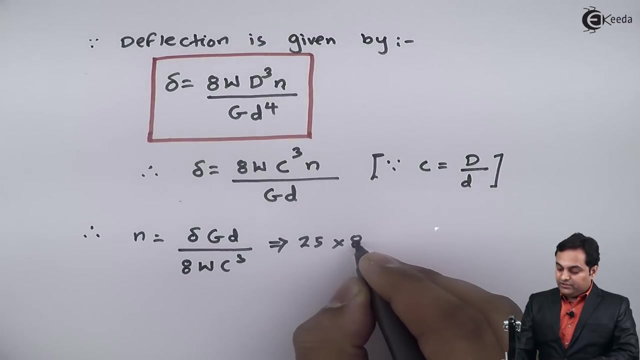 is the number of active coils. so n will be equal to deflection. this G D term will go onto the left hand side and in the denominator it will be 8wc3, so putting the values here, deflection it was given in the problem as 25 g- it was 84 into 10. raise to 3 small d. 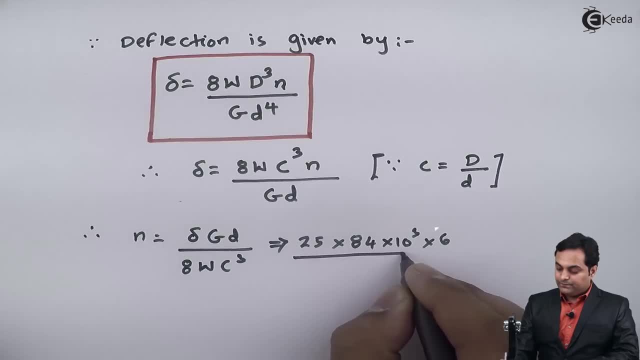 value we have calculated it is 6 upon 8. into w 500 c it was 8 cube. so from this, if I calculate, I will get the number of turns as 6.15, which I can round it off to. 8 means 8. number of. 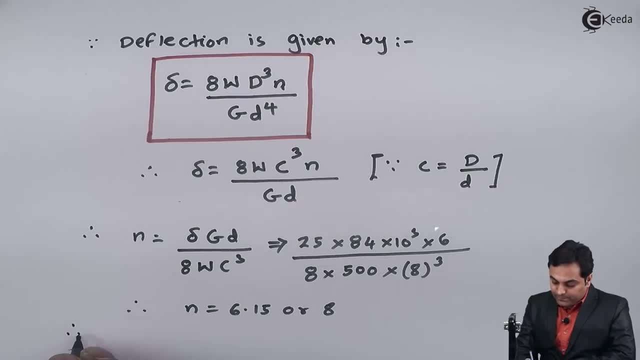 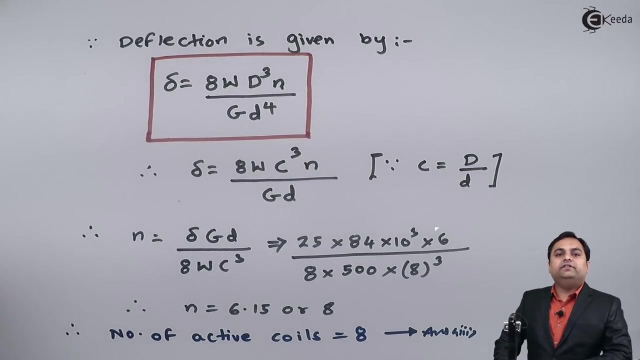 active coils are required. so I will say that, therefore, number of active coils is equal to 8. so here, after getting the values of wire diameter and mean coil diameter, the next value is number of active coils. this is our third answer. now, number of active coils means those coils which take part in the deflection. apart from this, there would be: 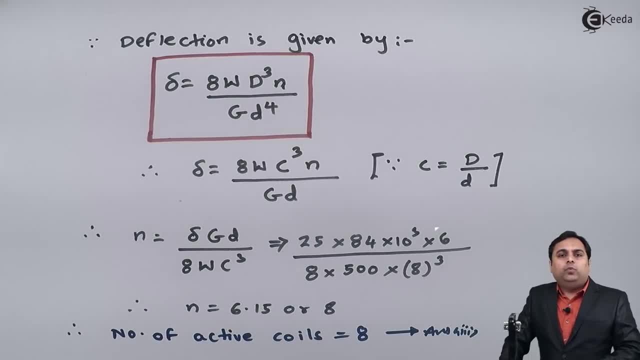 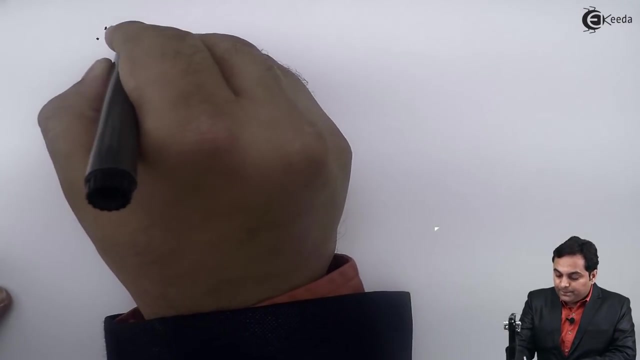 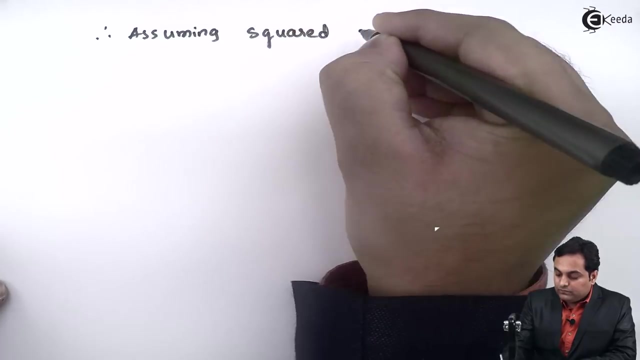 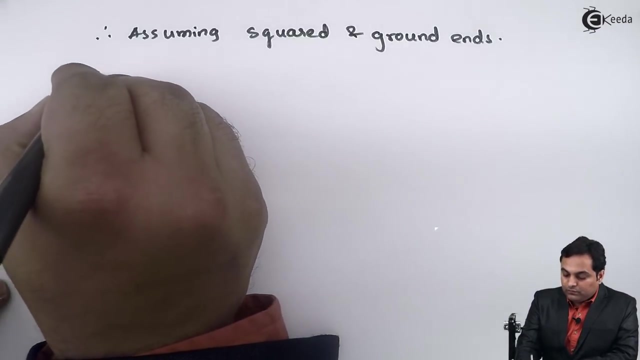 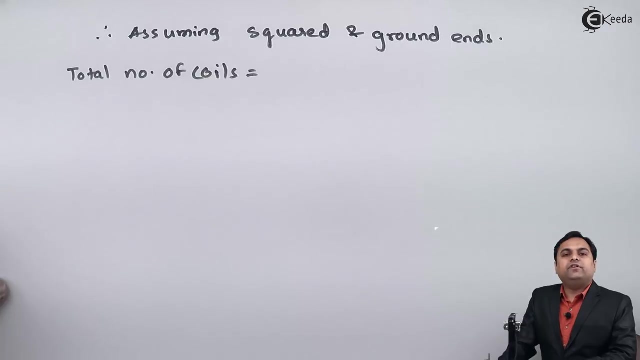 one coil at the top and another at the bottom which do not take part in the deflection. so here I will find out total number of coils. therefore I will write down: assuming squared and ground ends. total number of coils will be equal to number of active coils, which is 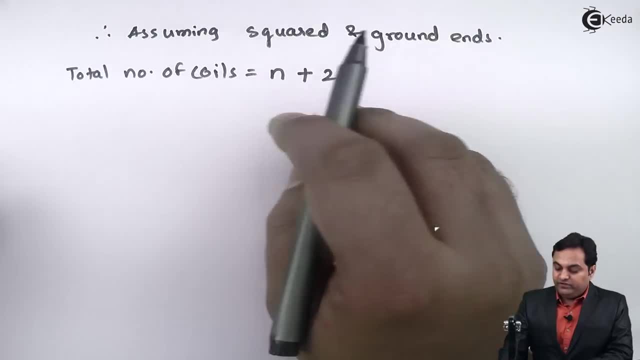 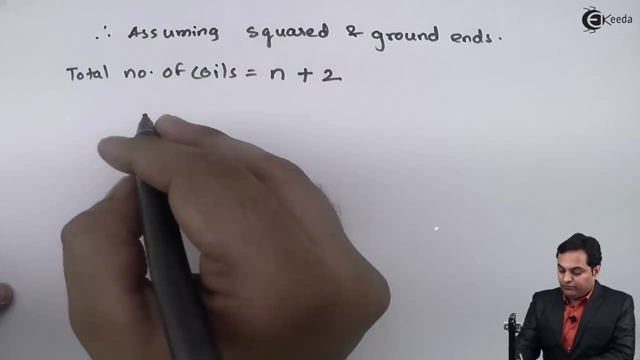 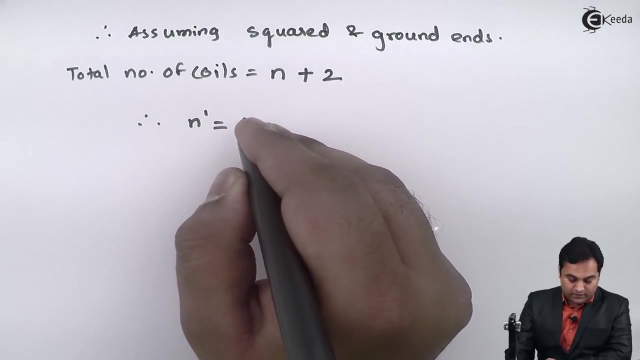 n plus two. when we are using squared and ground ends, then the total number of coils would be n plus two. therefore, total number of coils would be n. direct number of coils from back to front. I'll denote it by n. dash is equal to n. it is 8 plus 2, so the total number of 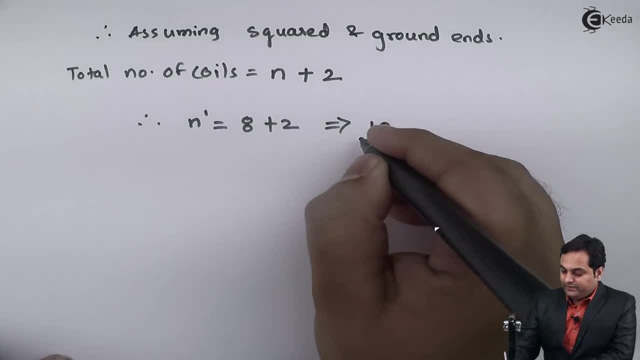 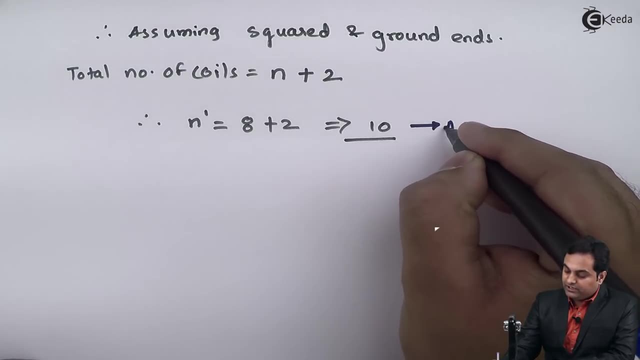 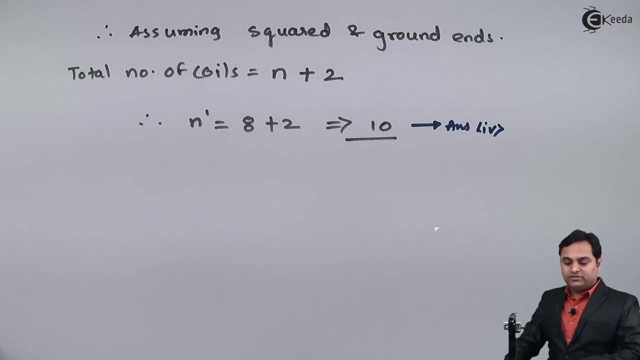 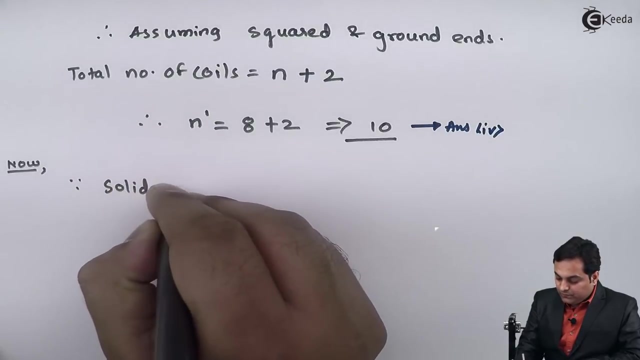 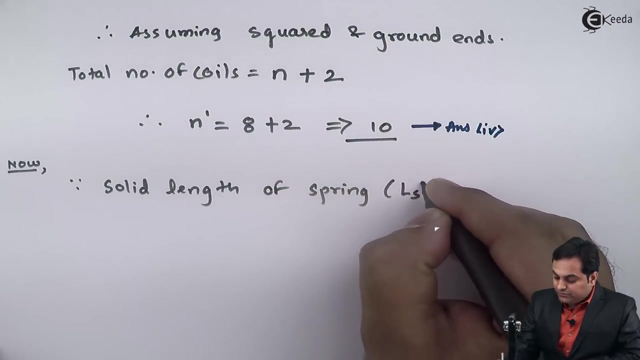 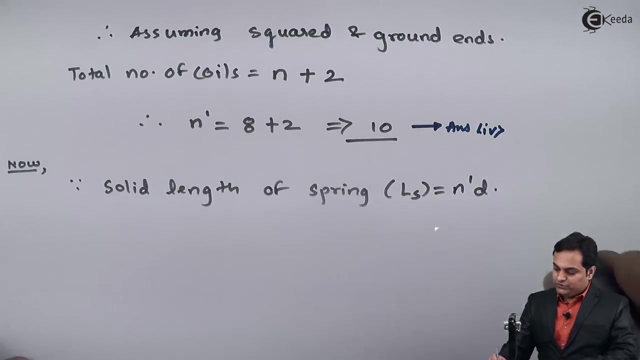 coils required are 10. next here I'll write down after getting the total number of coils. this will be the fourth answer for us, next after getting the total number of coils. now I can say that since solid length of spring, solid length is denoted by L suffix s, and that is n dash multiplied by the diameter of wire. so 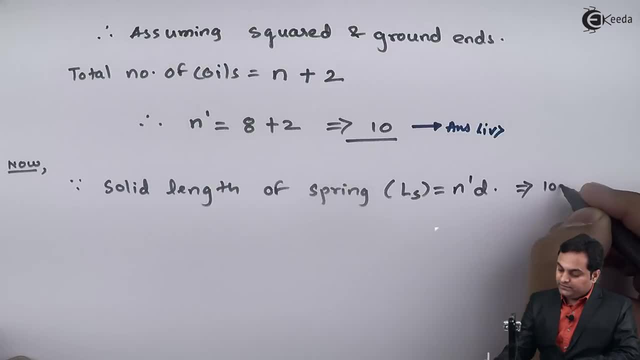 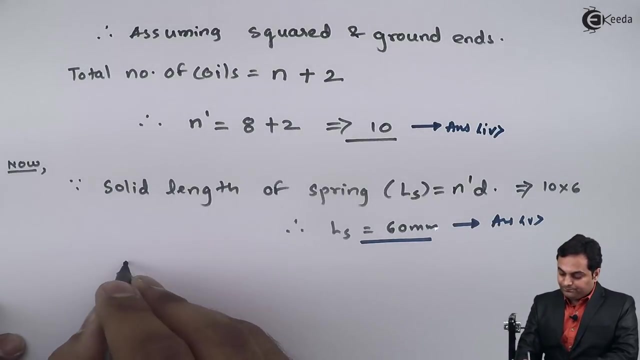 here we have n. dash is 10, diameter of wire is 6, so therefore solid length becomes 60 minus 10. so this is the total number of coils required to get the total number of coils, millimeters solid length. I can explain it with the help of a diagram. 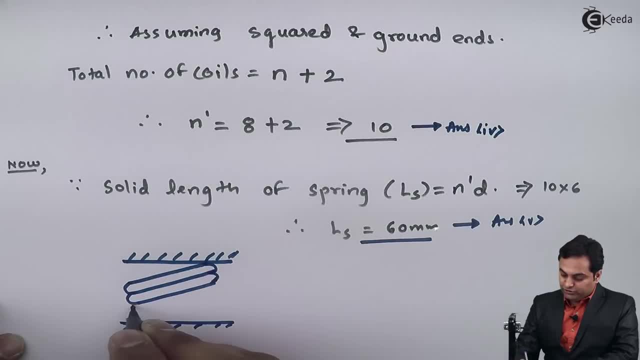 here I am drawing the diagram for solid length now. this solid length indicates that this solid length indicates that thewarz's diagram of linear préc giving length 20 millimeters is n dash, and then sl n dash is n dash, then sl n dash is n dash, and then 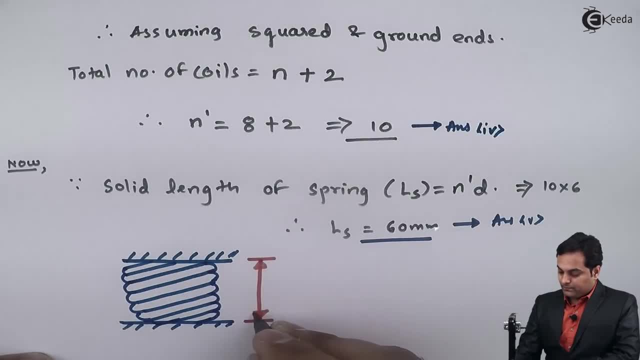 so this solid length. I can explain it with the help of a diagram. now, this solidお respuesta. nicely, this is the length of the spring in completely closed condition, that is, when we are applying the load. this spring would be compressed under the action of load, since we are using, or we are designing, the helical compression spring. 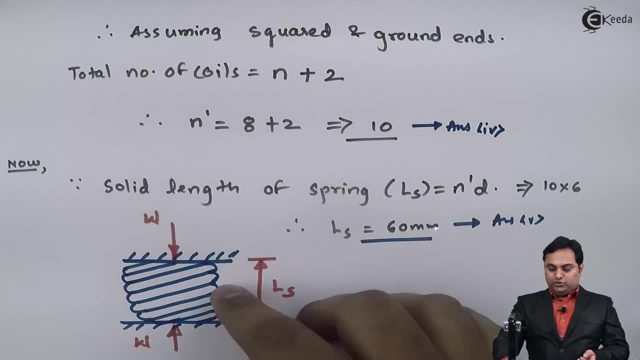 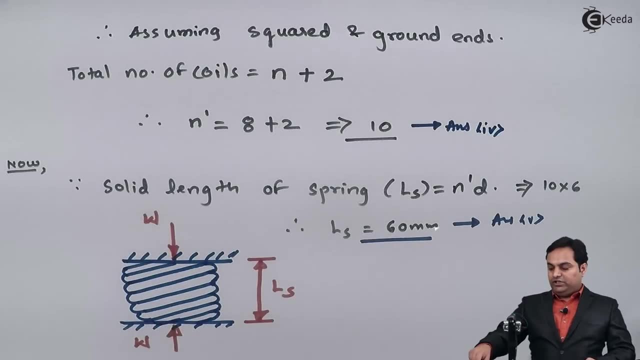 so when the load is applied, and then there should not be any gap between the turns of the spring or coils of the spring. so when it is completely closed, each of the wire diameters they are in contact. then this complete length would be called as a solid length of the spring. so while designing we should even 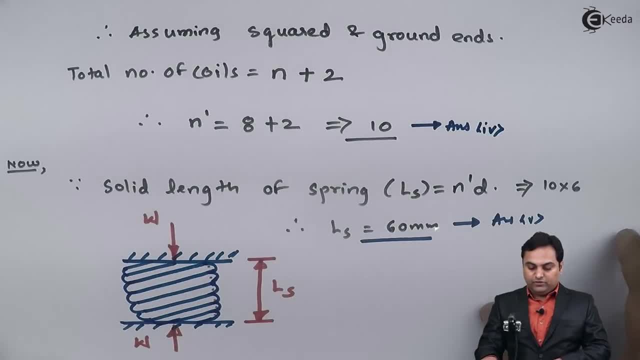 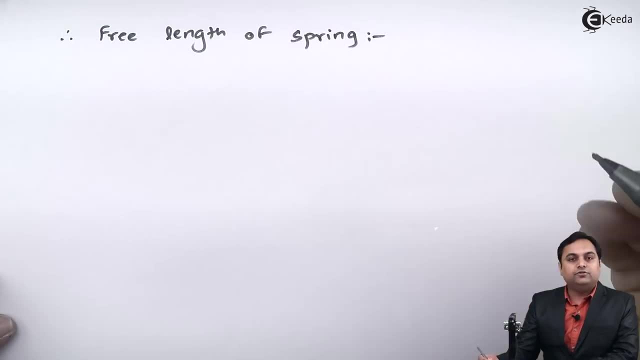 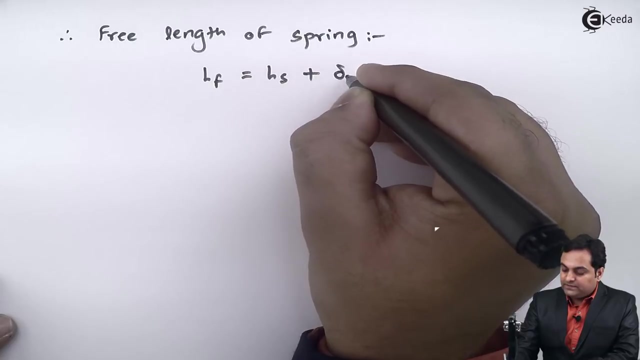 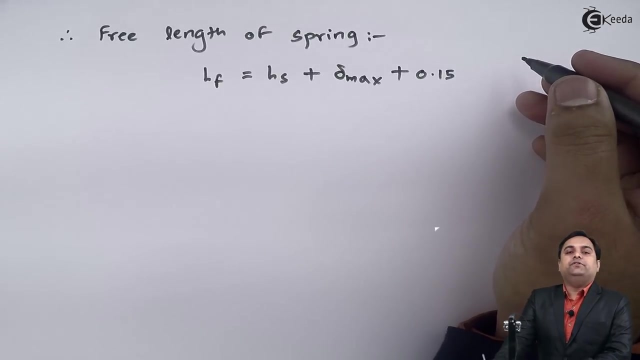 know how much should be the solid length. next I will calculate free length of spring. free length of spring, that is LF, is equal to solid length plus maximum deflection plus 15%. if I write it in the form of number, it is 0.15 of maximum. 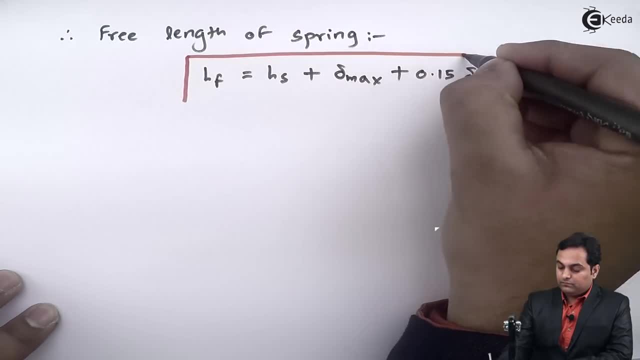 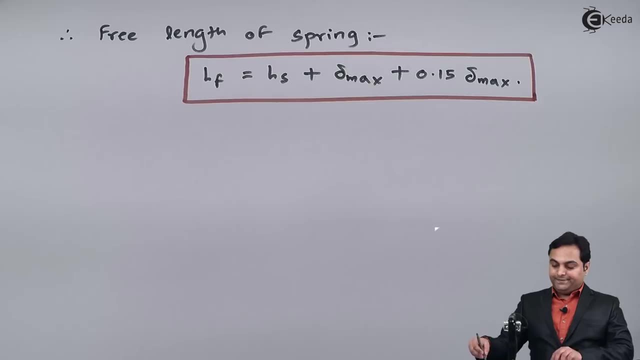 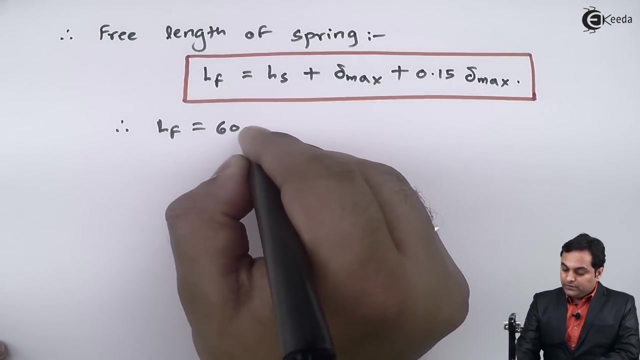 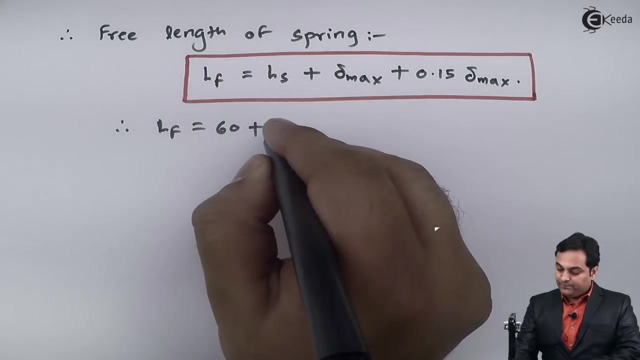 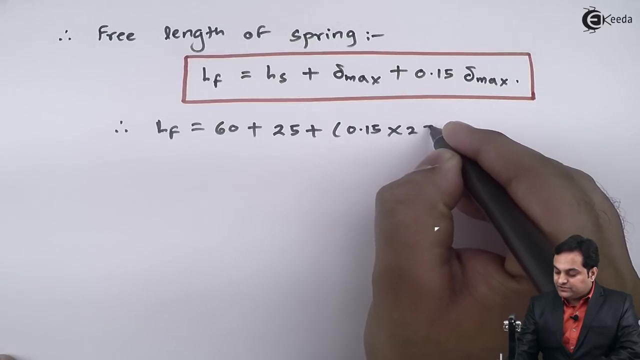 deflection. so this is the formula to calculate the free length of the spring. I'll go on putting the values. LF is equal to solid length is 60. maximum deflection is given in the question. it is 25 mm. yes, it is 25 plus 15% of maximum deflection, which is 25, and 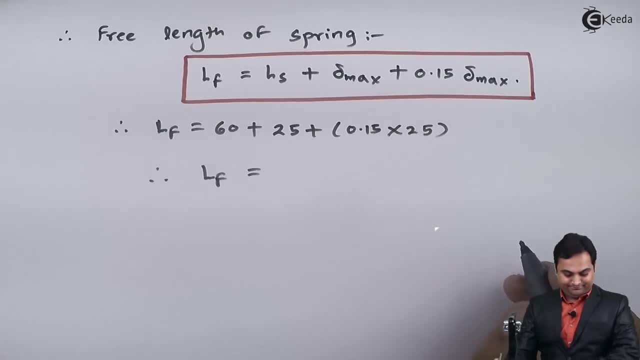 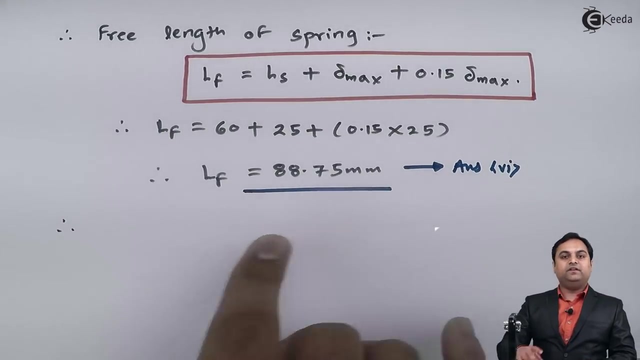 so my answer of free length it comes out to be 88.75 mm. this will be our sixth answer, after getting the free length of the spring. next I can calculate the pitch of spring. so after this I'll say that. therefore, now, before going on to pitch of the spring here, I'll explain what is free. 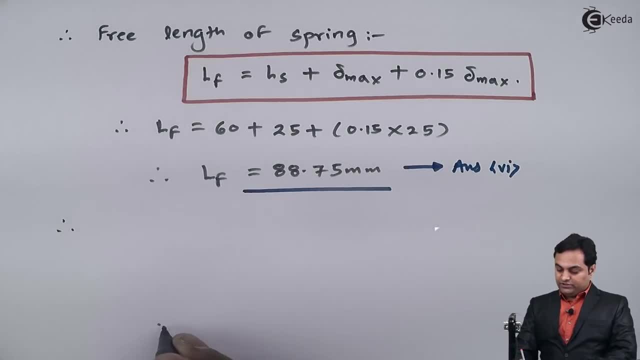 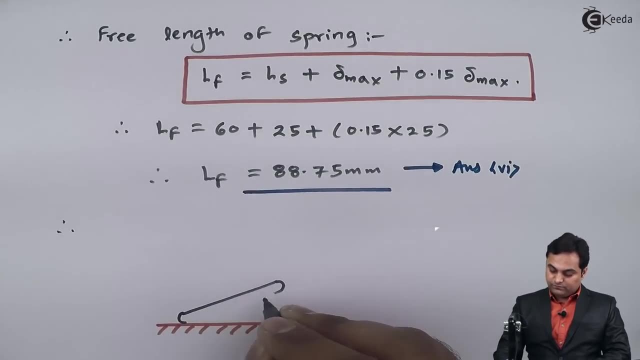 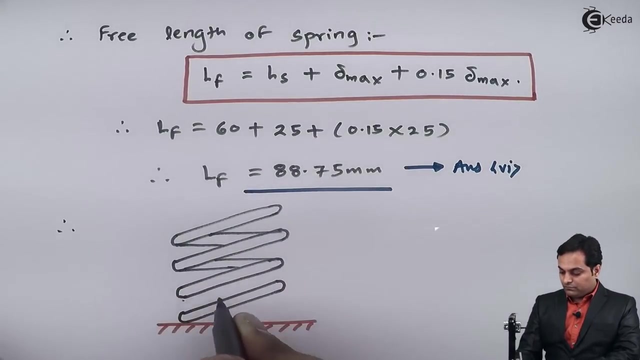 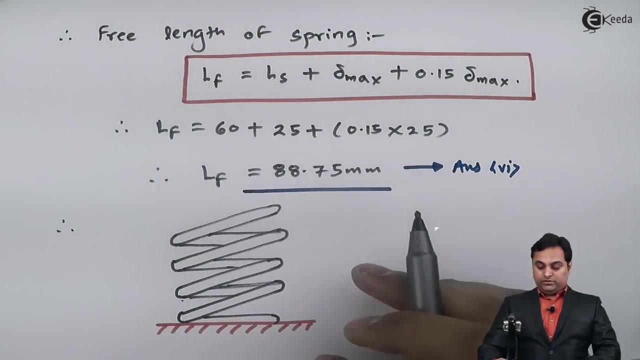 length. I'll explain what is the meaning of free length before going on to the pitch of the spring. here I am drawing the diagram for the free length of spring, explaining what it is. here I am drawing the diagram for the free length of spring. now the length string in the unloaded condition. 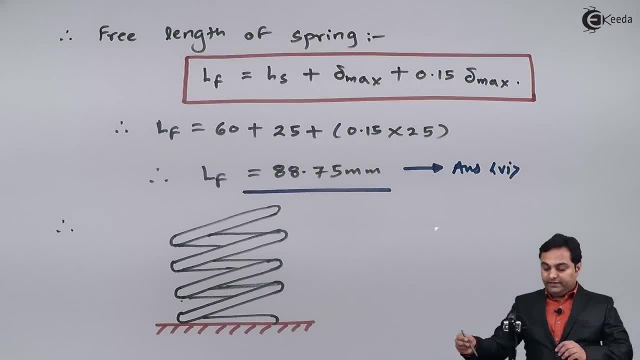 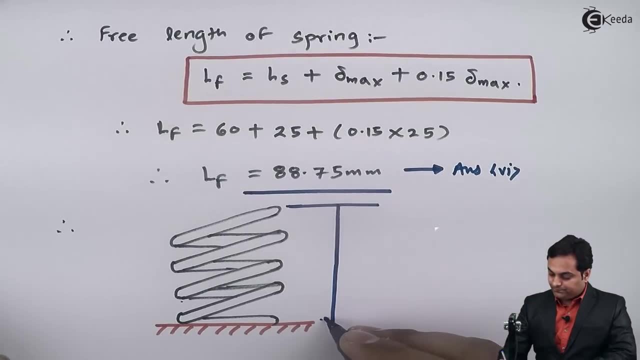 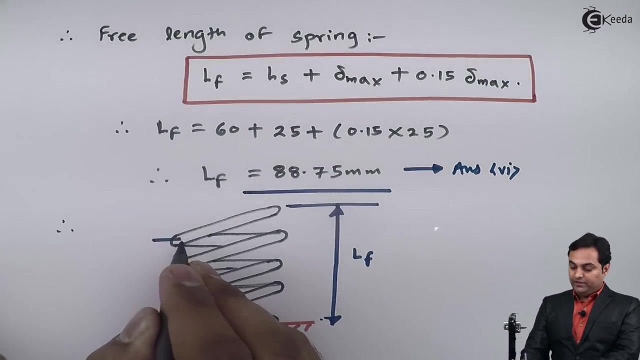 now the length spring in the unloaded condition, that is, when it is not loaded, then that indicates the free length of the spring. So here this complete length is the free length of the spring and maximum deflection it would be. we can measure it from the total we are getting, the deflection at each of the ends. 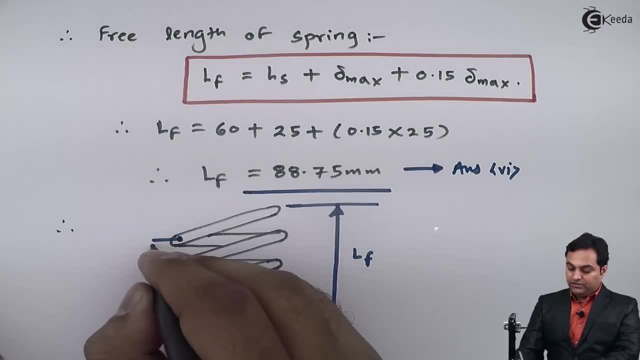 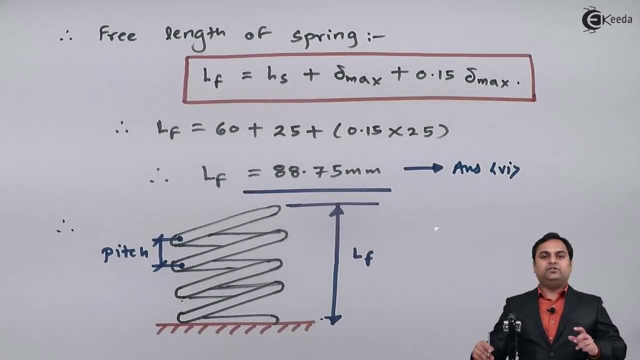 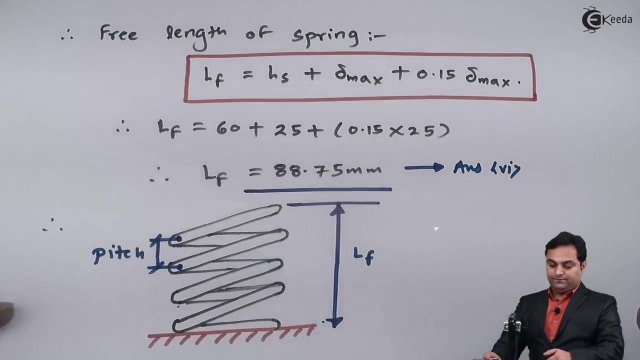 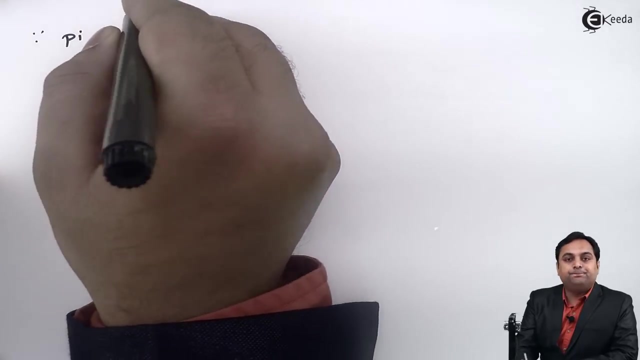 so that would be the maximum deflection. and here is the pitch. So free length indicates the length of the spring in the unloaded condition. Now, after getting the free length of the spring, the next thing which we have to calculate. it is the pitch. So it is called as, since pitch of coil. 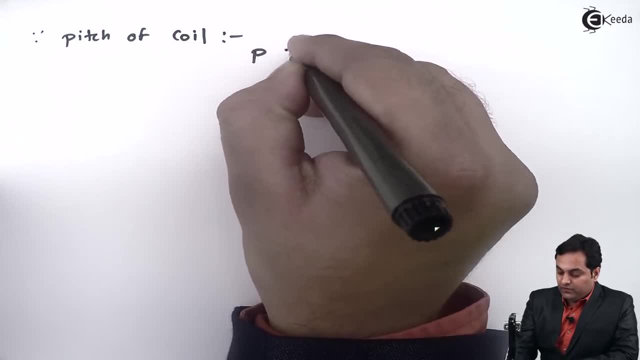 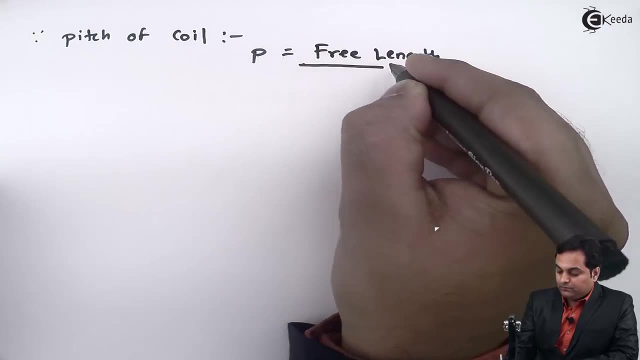 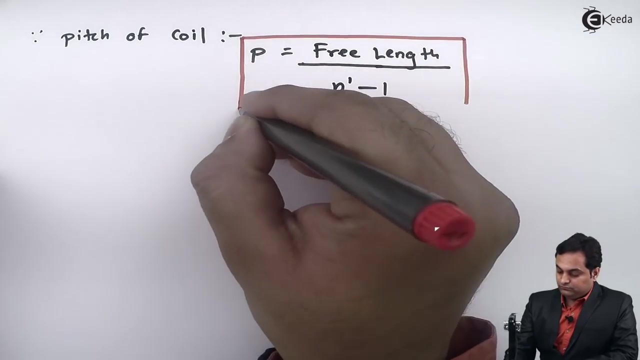 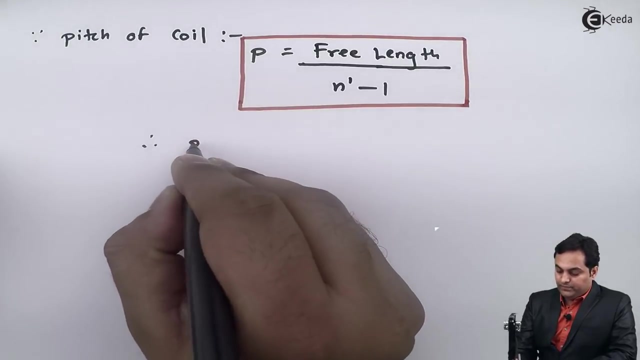 So, Which is p is equal to. the formula is free length upon total number of coils, which is n-1.. From this formula we can calculate how much is the pitch. So therefore, pitch will be equal to: free length is 88.75.. 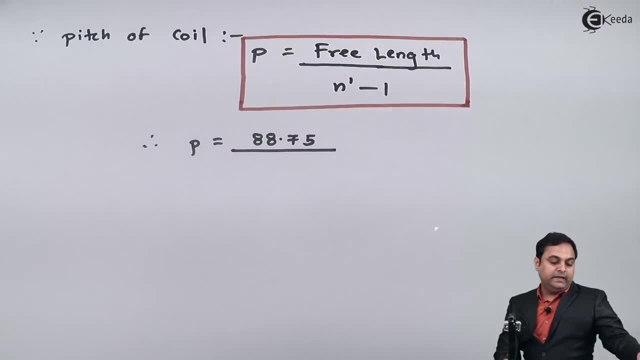 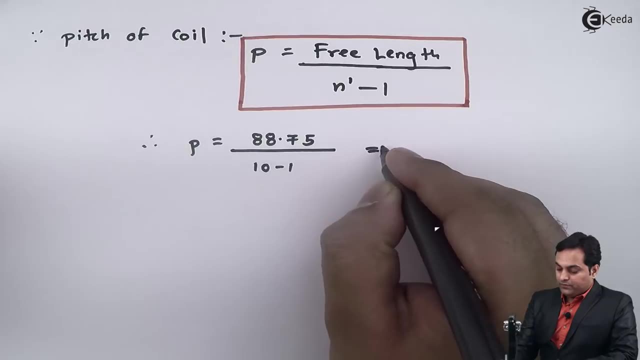 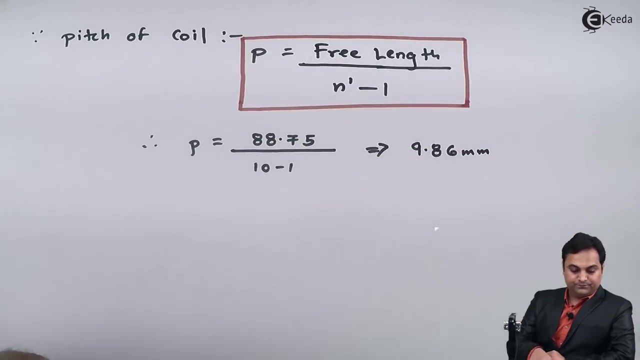 So Upon n-1, n-1 was the total number of coils and the value was 10.. So 10-1. so here pitch comes out to be 9.86 mm. This is the seventh answer for us Now, after we have reached up till pitch. next I'll say that whatever 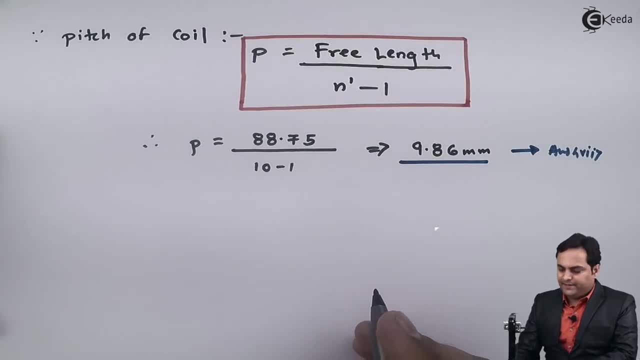 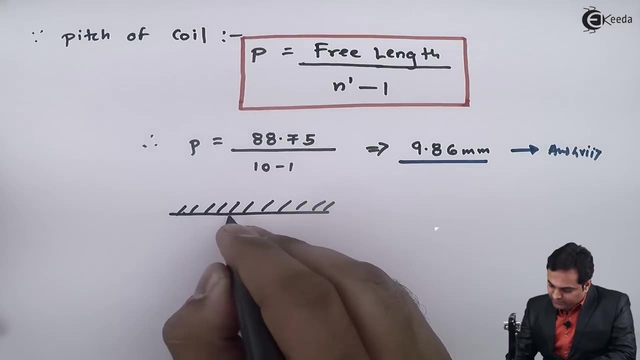 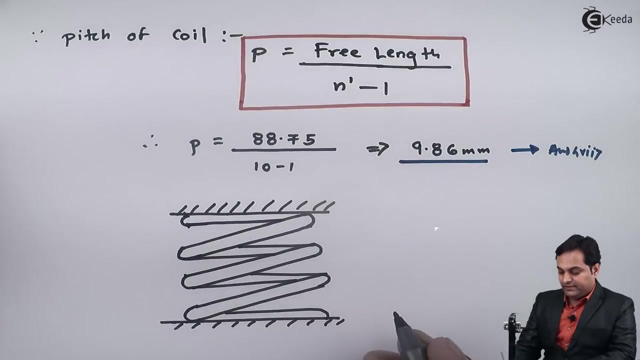 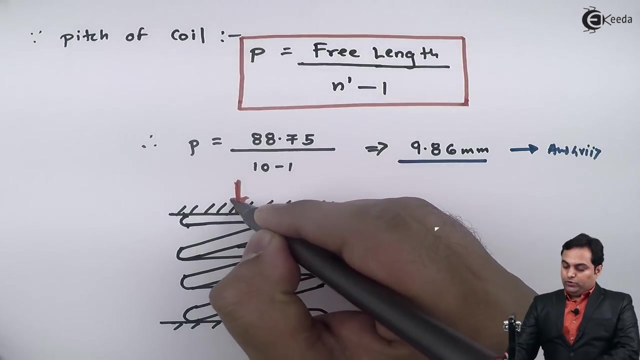 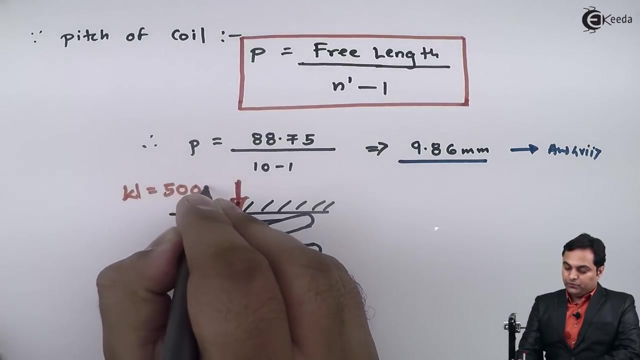 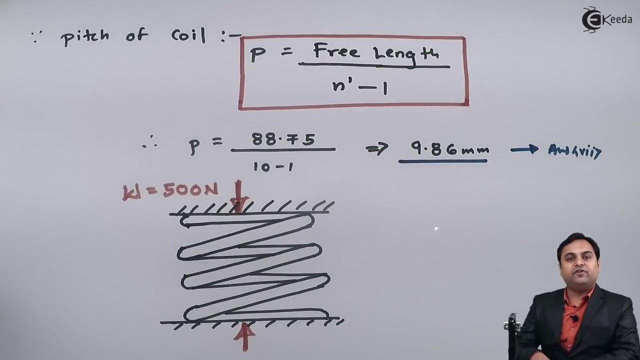 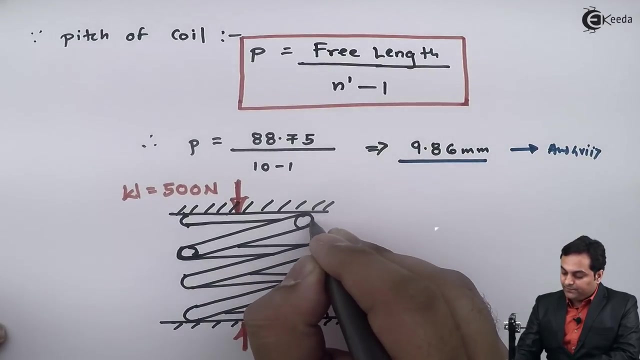 Dimensions we have found out. I will denote it on a diagram. Here I am again drawing a helical compression spring. This is the diagram for the helical compression spring. Here I have drawn the diagram. Now this indicates a helical compression spring When we are applying load over. this load is given in the problem. It is 500 Newton. So under the action of 500 Newton load this spring will compress. And here the first thing which we have found out was the wire diameter. Wire diameter is a small diameter here, with the help of which the spring is made. 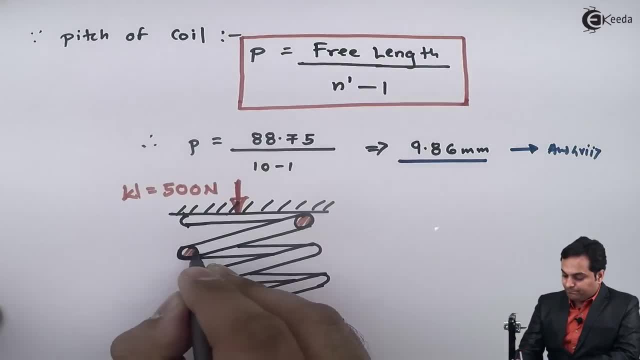 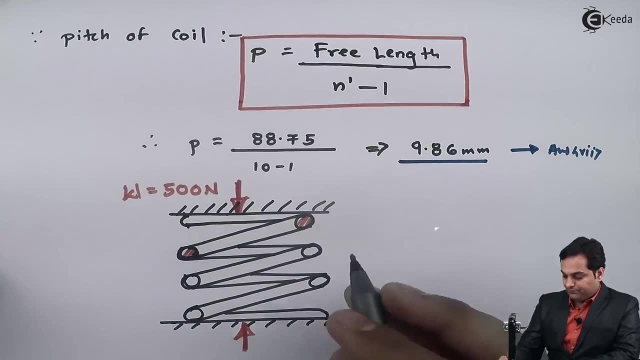 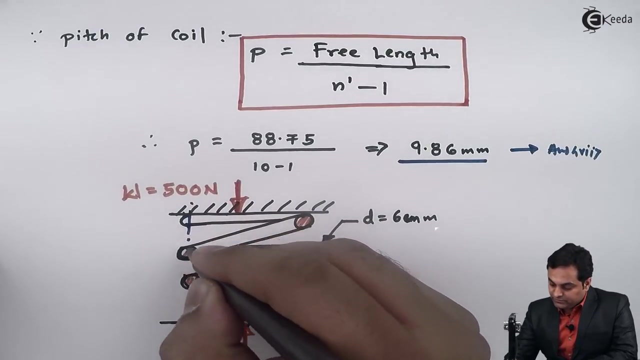 It is this diameter. These are the wire diameters. So here in this problem we have got the wire diameter as small. d is equal to 6 mm, Then the mean coil diameter is equal to 6 mm. Here that is the line which is passing through the center of this wire on both the sides. 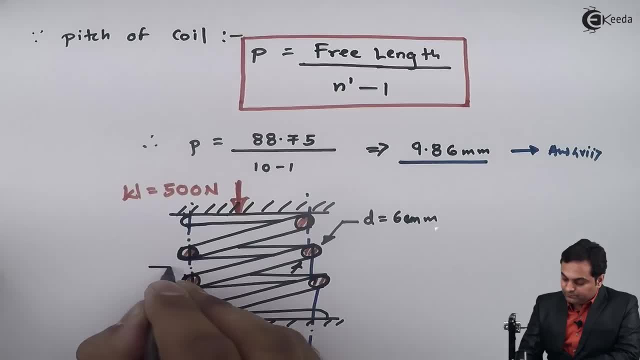 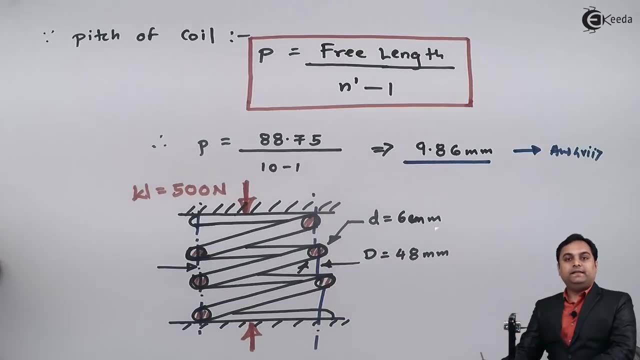 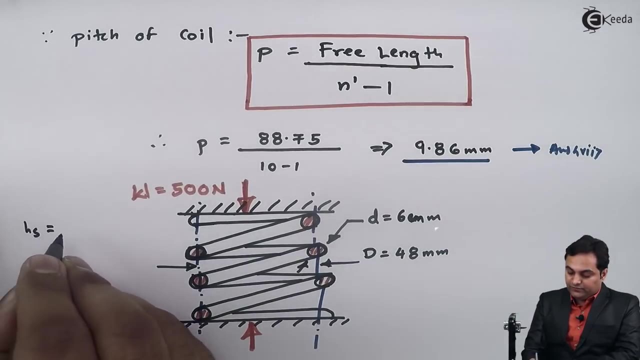 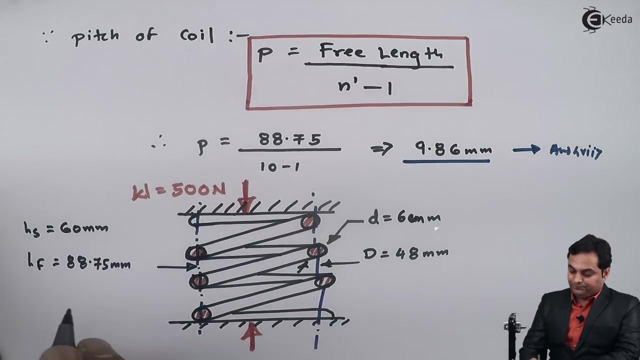 This was the mean coil diameter And it was 48 mm. Next, after this, we have calculated the solid length. Solid length was 60 mm, Free length of the spring that was 88.75 mm. Then, after getting solid length and free length, we had calculated the number of active coils, which was n equal to 8.. 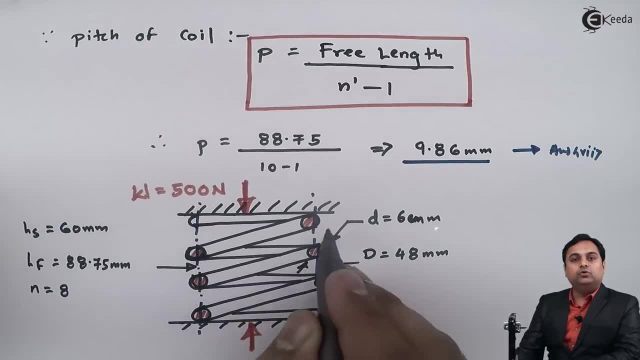 Active coils. are these coils which are subjected to compression or which take part in the deflection. Apart from that, we have 1. And 2. These 2 turns of coil which do not take part in the compression because they are fixed.